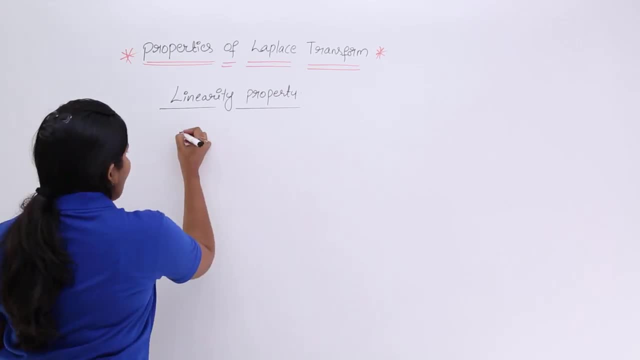 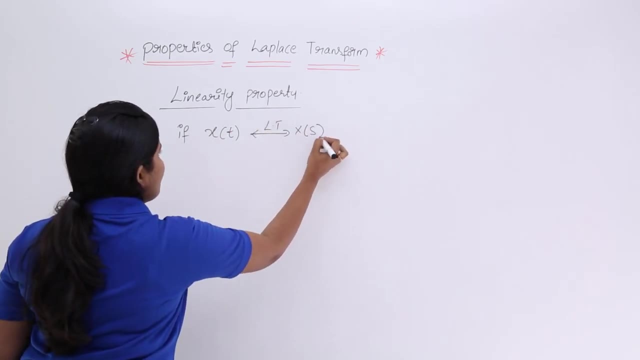 I want to consider two signals. So I want to consider x of t for this, if Laplace transform is x of s, and I am considering another signal, y of t, for this, the Laplace transform is y of s. So these two signals I consider to explain the linearity property in Laplace transform. 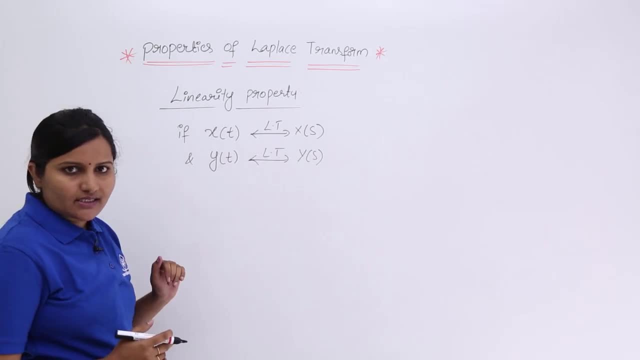 So if a signal x of t is having Laplace transform x of s and y of t is having Laplace transform x of s, then I am considering the linearity property of Laplace transform. If you added these two signals and take in transform, how they transforms are related. 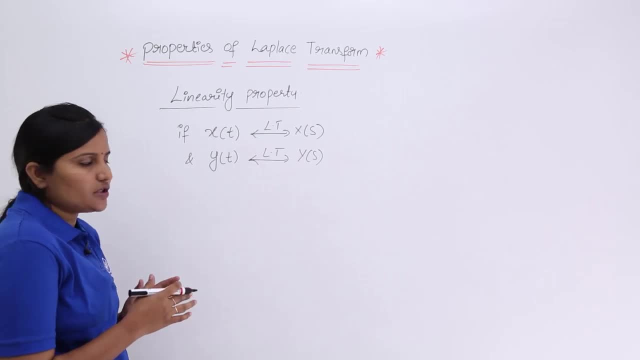 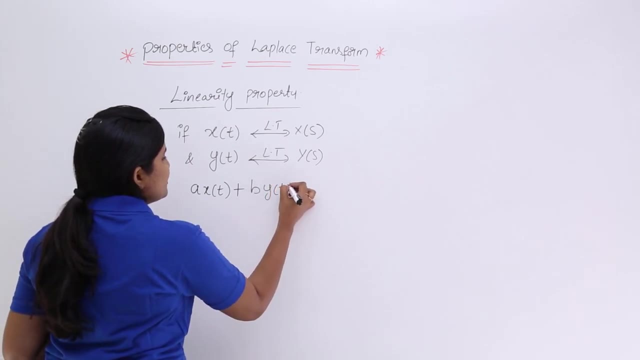 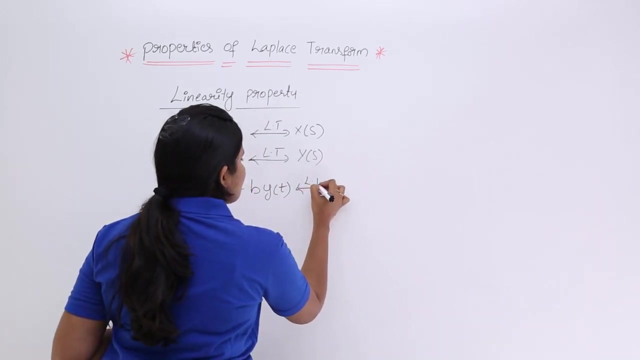 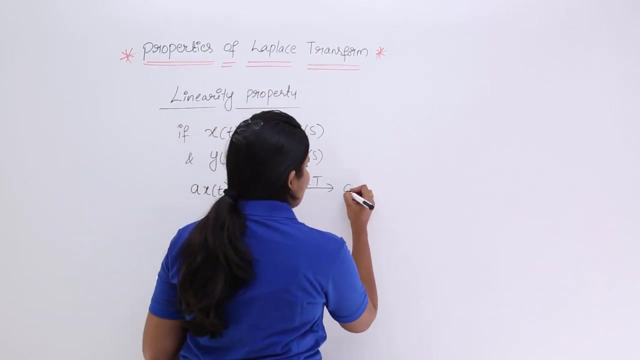 means those are also similar to our signal modulation. That means, if you calculated signal like this, that means if you consider the addition of these two signals like this, for this combined signal, if you want to calculate Laplace transform, if you want to calculate Laplace transform for this combined signal, this will be- is equivalent to combination of individual. 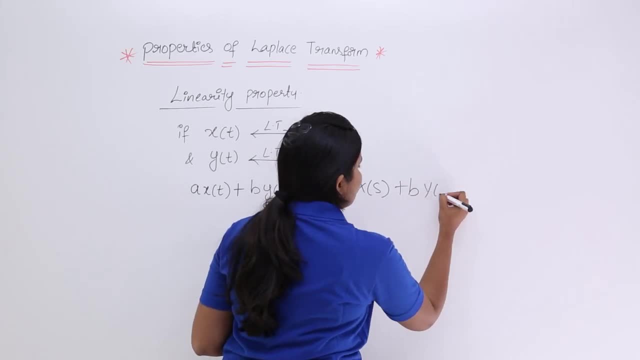 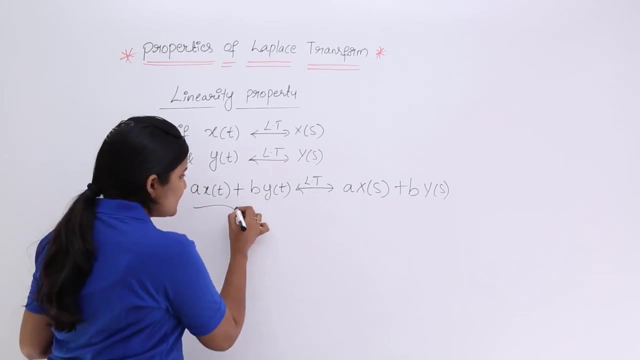 transforms similar to combination of individual transforms. That means a into x of t plus b into y of t. this is a resultant signal. x of t is a signal and y of t is a signal. by combining these two signals you will get a different signal in practice. If you consider Laplace transform of 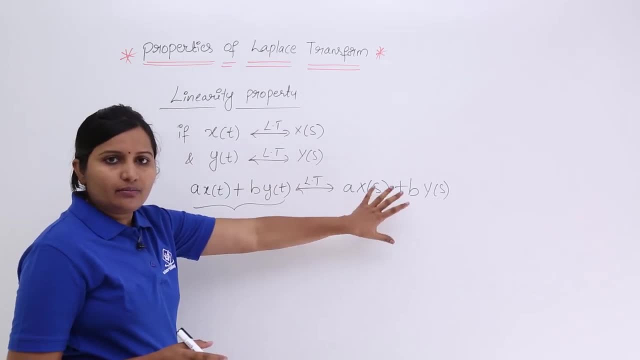 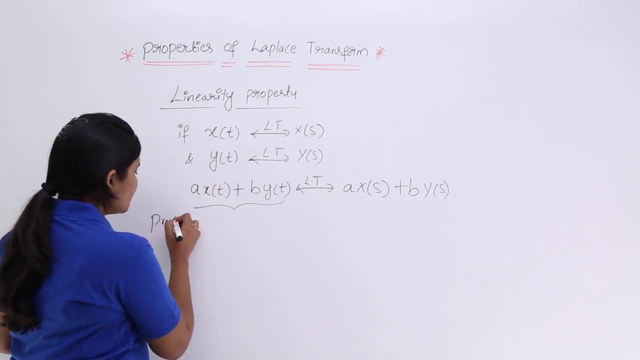 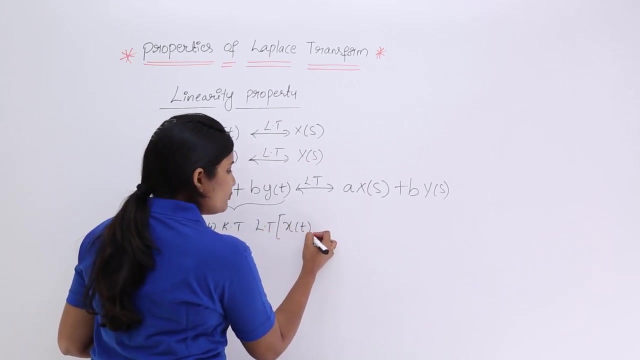 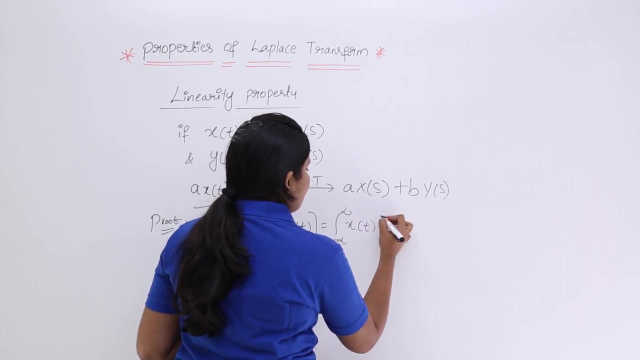 that signal, then you are going to get same like addition of individual transforms. So now here I want to prove this. We know that. we know that Laplace transform of x of t is equivalent to. we derived this formula integral minus infinity to infinity x of t into e power. 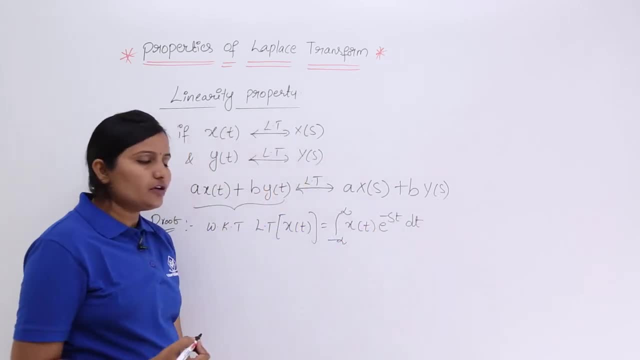 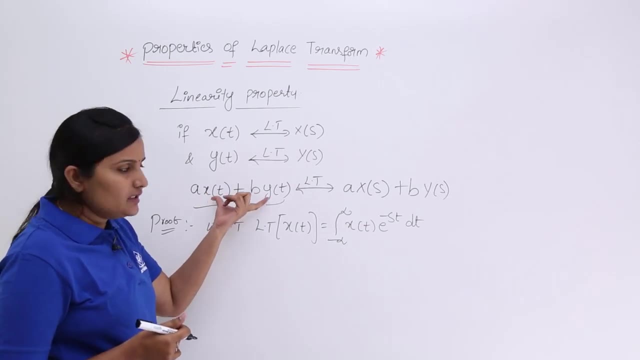 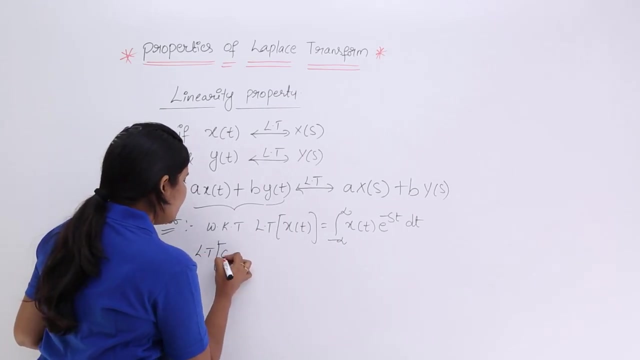 minus s, t, d, t. This is the equation for calculating Laplace transform For any of the signals that is involved. in favorites you should take the laplace transform as the differential result Here, room resultants and we will see that Einspanner Quiz. Let me come over an example that makes sense for evaluation of this particular problem. 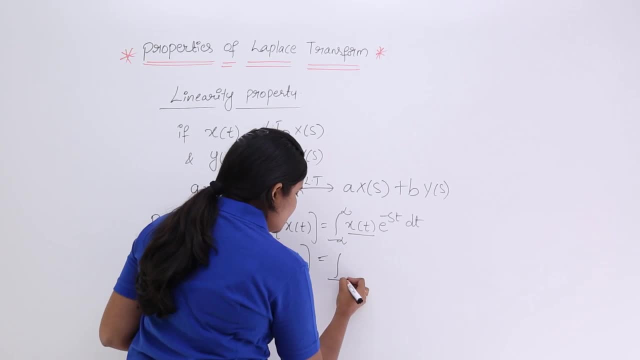 This last five only short problem will include the quand marks in a particular group of the four segment, bile How to identify Hai gangこうkopiao which may beijnest in these rotors of the society variables in combination of chi, poplar d, pase, C and xb and u and x. This is a very simple question. But you need to prove here for this resultant signal, this is the Laplace transform. So here I am considering that Laplace transform of a into x, of t plus b into y, of t is equivalent to. we need to calculate this. so in place of this signal I am substituting this combined signal. That means integral. 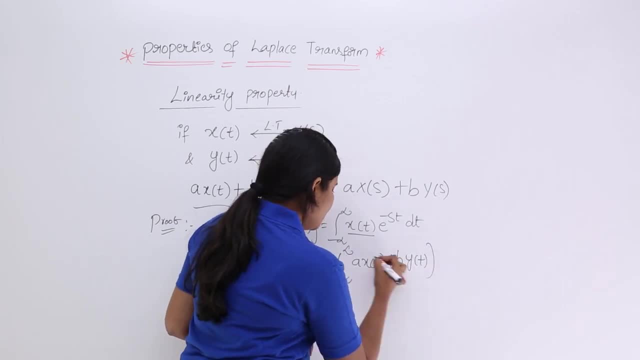 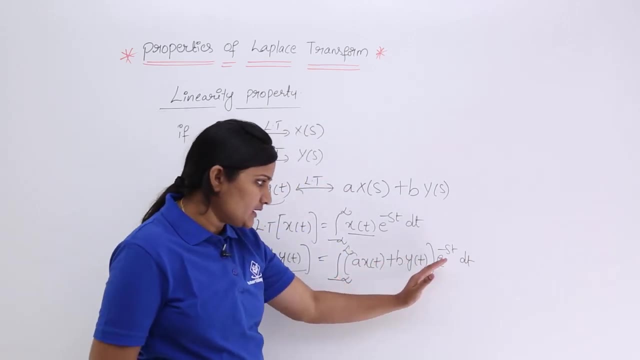 minus infinity to infinity connections, or networkρόph plus b into y of t, into e power minus st, dt. Here I am expanding this e power minus st. I am separately multiplying this e power minus st to both x of t and y of t. in the next step, 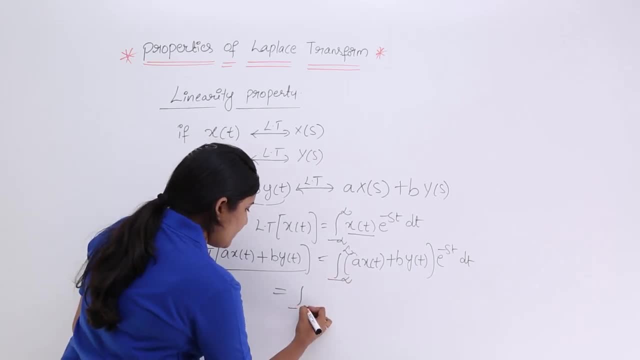 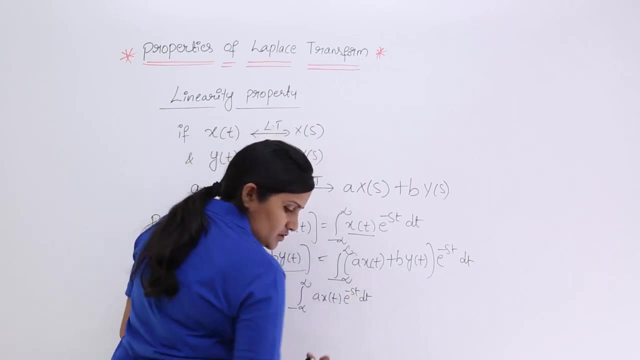 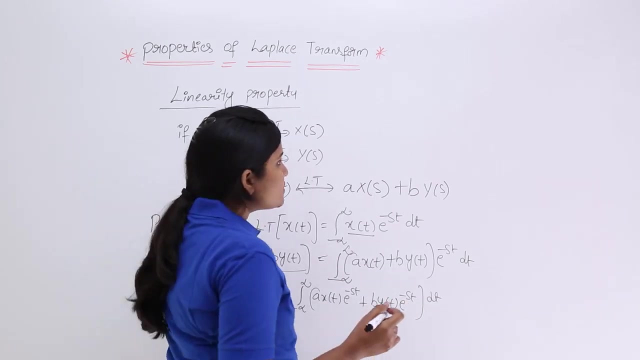 So here this is equivalent to integral minus infinity to infinity: a into x of t e power minus st, dt plus. So here: a into x of t e power minus st plus b into y of t, into e power minus st dt. So I am separating integrals to both this factors. So now this is equivalent to: 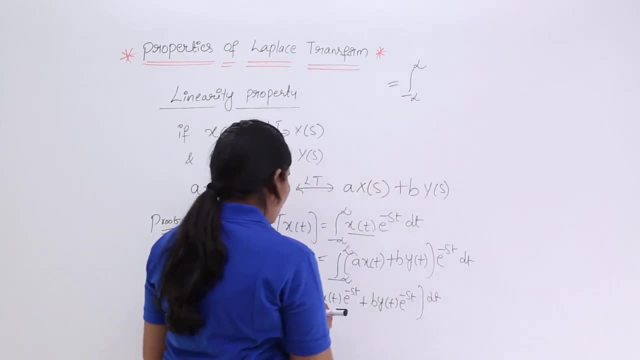 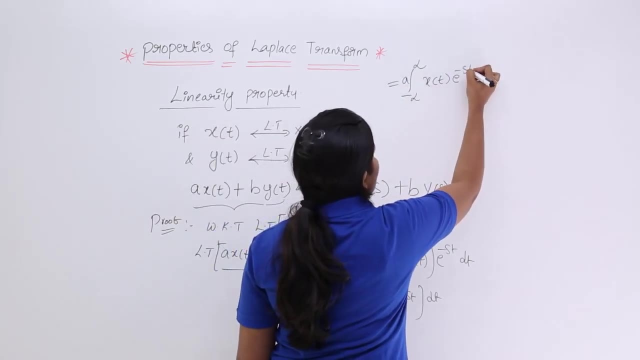 integral minus infinity to infinity. So here I am taking common of this a and here x of t into e. power minus st dt. So here I am separating integrals to both this factors. So now this is equivalent to integral minus st dt, plus I am taking this integration to this factor and here 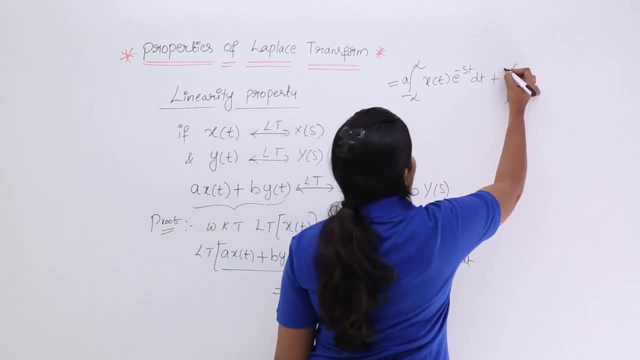 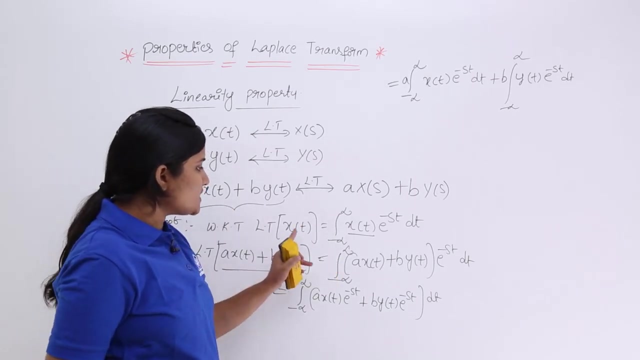 this b is common here because that is a constant, and b into y, of t, into e, power minus st dt, So minus infinity to infinity. Here, if you observe these two formulas, these are similar to Laplace transform equation. Laplace transform of x, of t is equivalent to x, of s is equivalent to So. 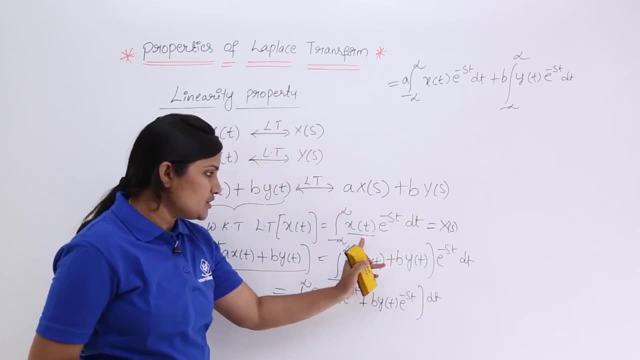 this is nothing but x of t. So this is nothing but x of t. So this is nothing but x of t. So this is nothing but x of s. So x of s is equivalent to integral minus infinity, to. 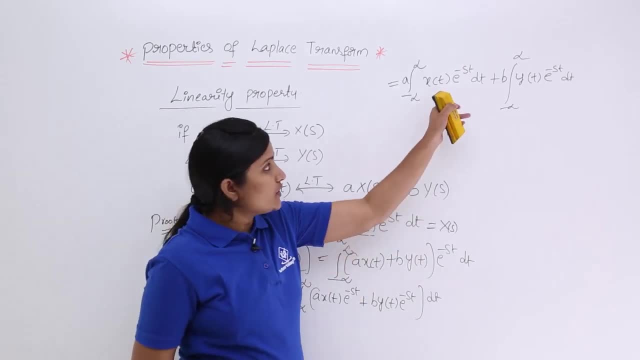 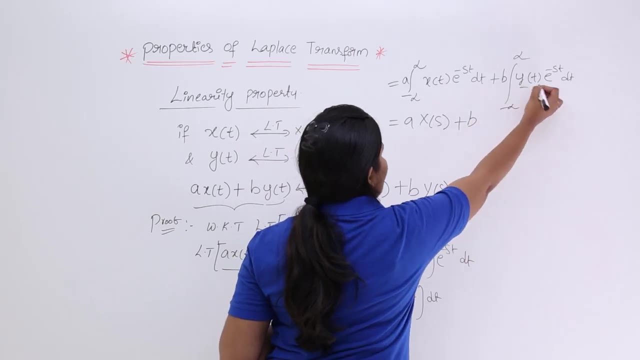 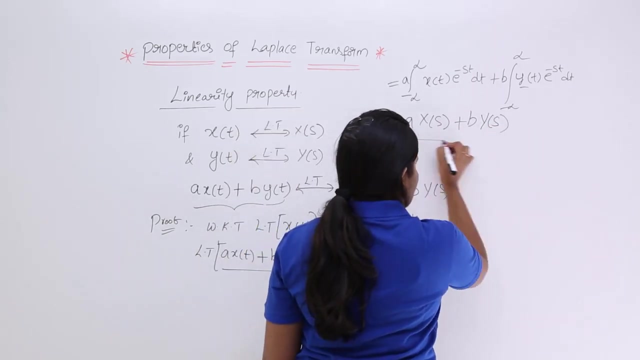 infinity given signal into e power minus st, dt. So if you see, here this is equivalent to a into x of s. Similarly, in the signal place if you are having y, means you are going to consider the Laplace transform of y of t, So that is nothing but y of s. Like this we can say for example: if anyone 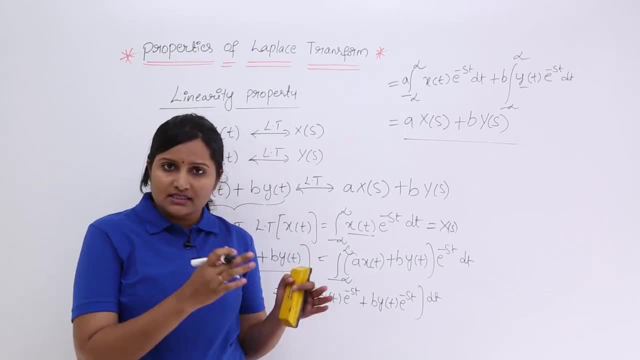 given you the spectrum of two signals, is this: So this is nothing but x of s. So this is nothing. but this is nothing but y of s. So this is nothing. So that is nothing but x of s. So this: 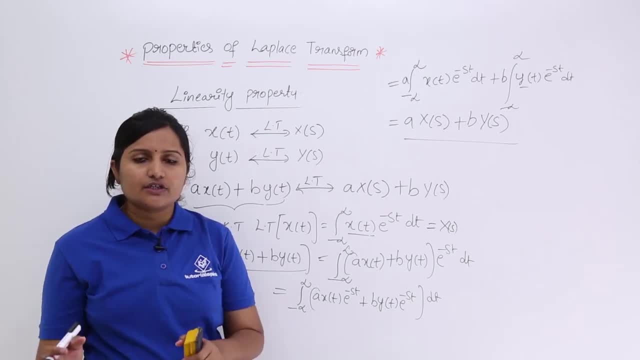 is nothing but x of s. So this is nothing and this They given this spectrum of two signals is x of s is equivalent to something and y of s is equivalent to something. Then what is the addition of time domain of that signals? If they are asking what is the addition, 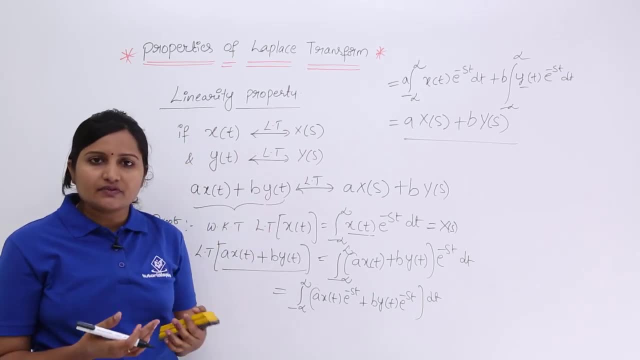 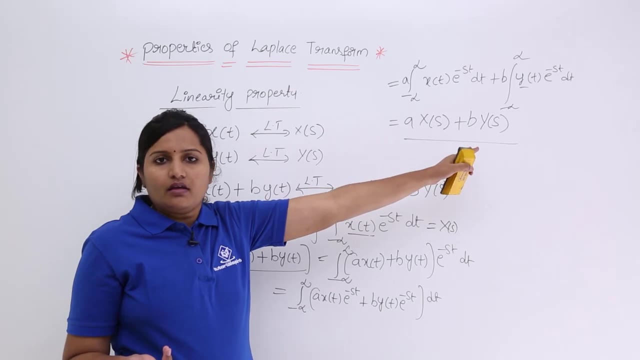 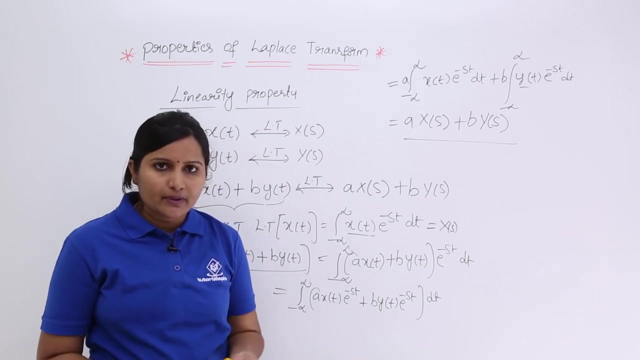 of time domain, of that signals. if they are asking, then how you will do means just you will take like this and you will take inverse Laplace transform, Then you are going to get this. So, like this way we need to use linearity property at the end of these properties. we 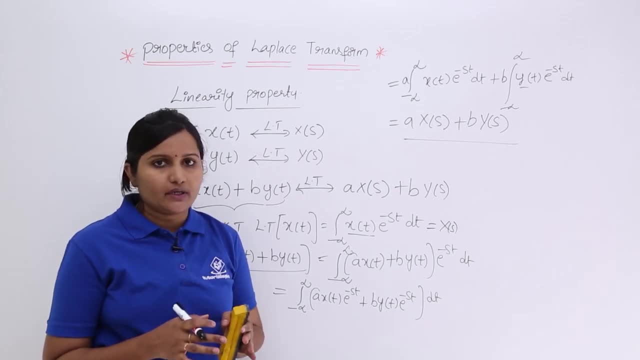 are going to solve some problems related to linearity property. In next few classes, we will discuss each and every property with proof. after completion of all these proofs, we are going to- ah, we are going to solve some problems related to this properties. 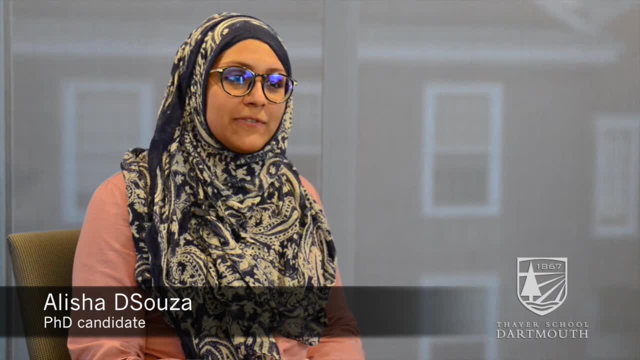 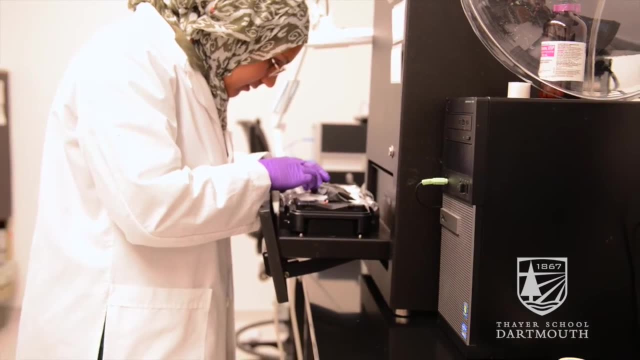 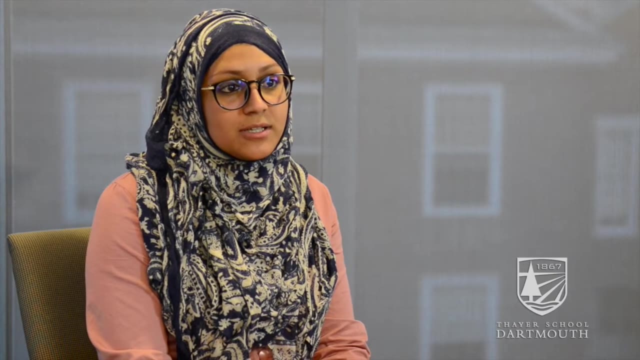 I'm Alisha D'Souza. I'm a fifth-year PhD candidate and I work with Professor Brian Pogue. My research involves using optical imaging and tomography methods to quantify the concentration of fluorescent molecules in tissues, and we use this to estimate tumor burden in lymph. 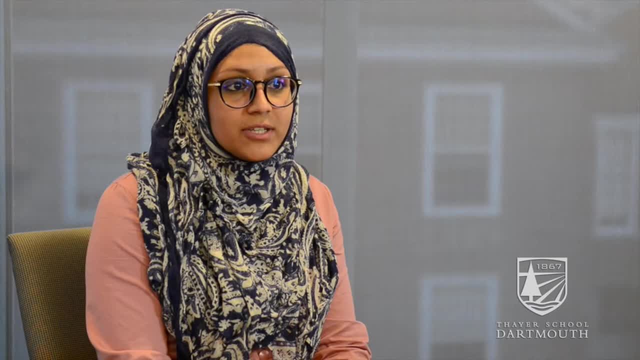 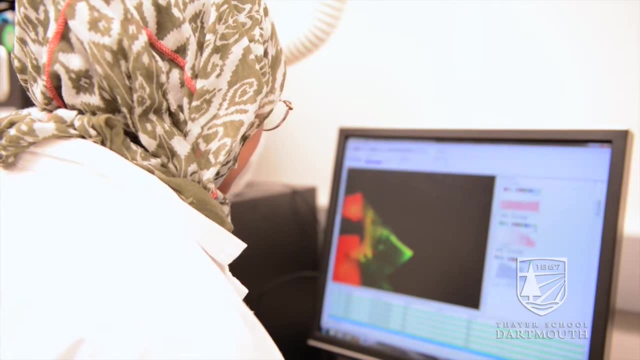 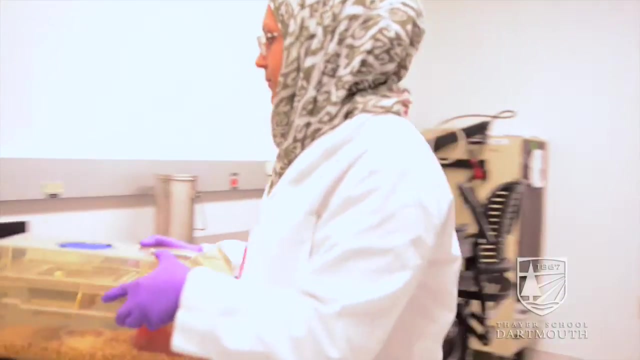 nodes, which allows us to non-invasively stage a cancer. A lot of my work has involved visualization techniques and experimental methods, where we develop models for cancer in animals. When I'm running experiments, what I usually do is we have animals or phantoms, which are basically 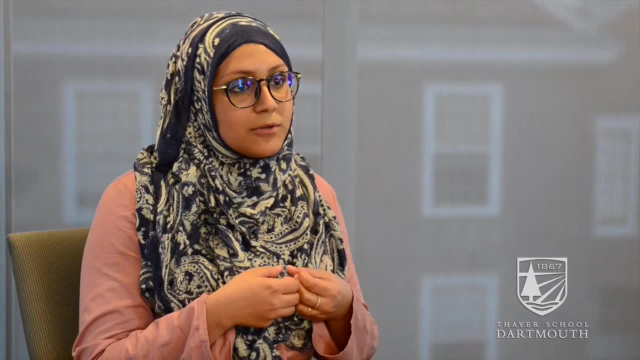 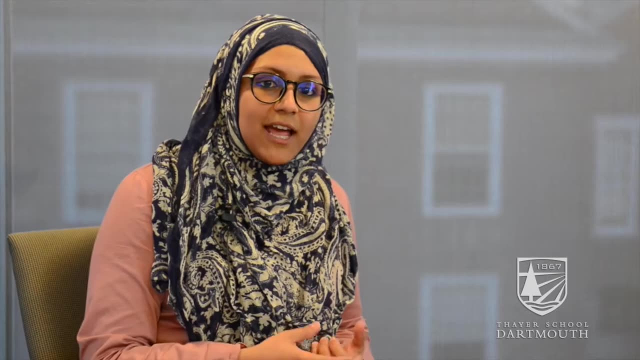 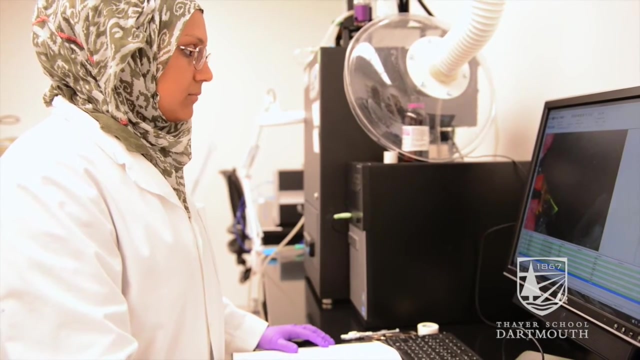 tissue simulations, and what we do is we either embed some fluorophores inside them or, if we're using animals, we inject a fluorescent dye at an injection site and have it get taken up by the lymphatic system and drain to a lymph node. I then use the video sequence. 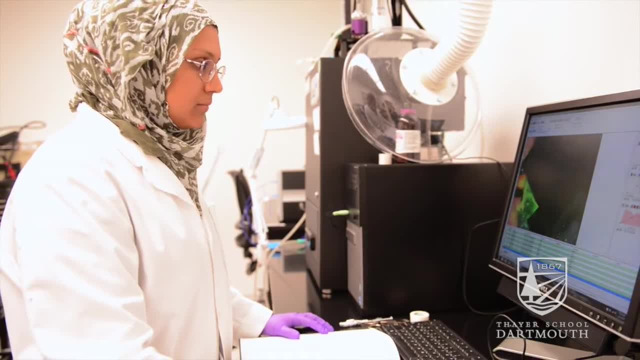 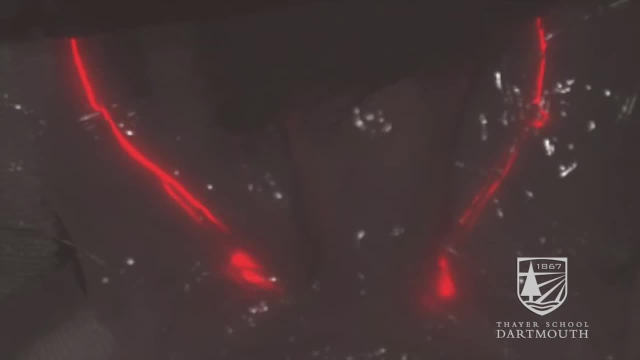 that I've acquired from these animals. Animals process that and then extract as much information as possible from it to get some quantitative estimates of the presence of cancer in the lymph nodes In a lot of major cancer types such as breast cancer, skin cancers and head and neck cancers typically. what happens is the cancer spreads by migrating through the lymphatic system of the body. They move through the lymphatic system and then get trapped in tissue bodies, which are lymph nodes. What is typically done in the clinic during the treatment of cancer patients is they locate the lymph nodes of interest.